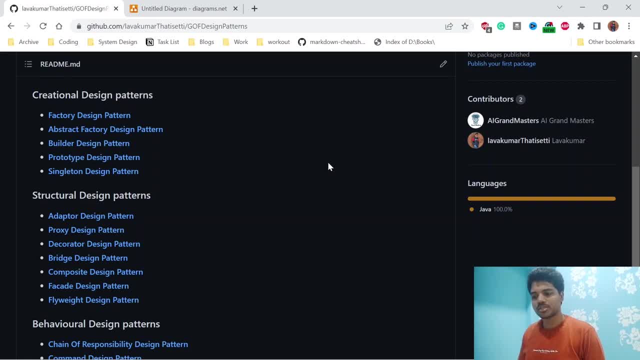 Hi, welcome to my channel. In this video we are going to discuss about composite design pattern. In my past videos I have completed creation design patterns and also top 4 structural design patterns. In the next three videos I will complete the structural design patterns also. 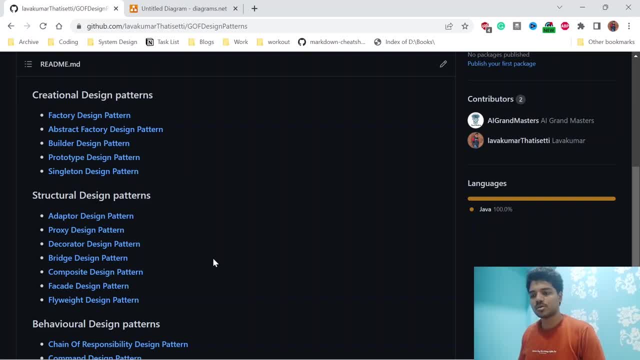 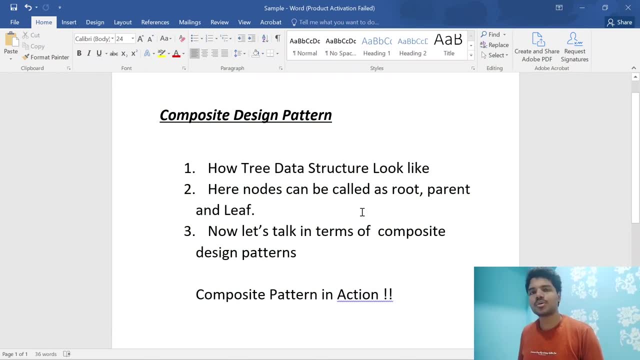 So if you miss the videos, please go and watch those videos. I will put the link in description. Now let's talk about composite design pattern. Before going into composite design pattern, let's understand how tree data structure basically look like. So what are the main components in tree? 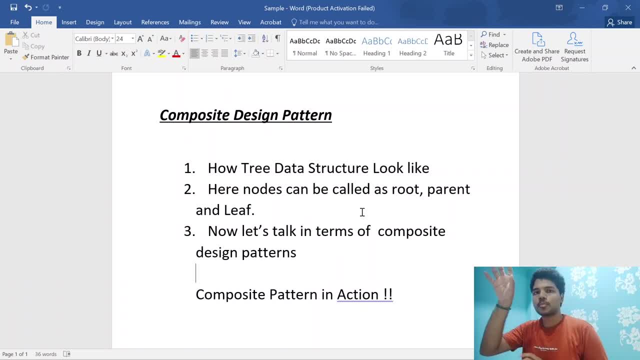 data structure. So tree has different set of nodes. Top node will basically called as root and also there are, like, childrens for the root and childrens will have sub-chails. So those childrens which have sub-chails will basically called as parents and those childrens which are 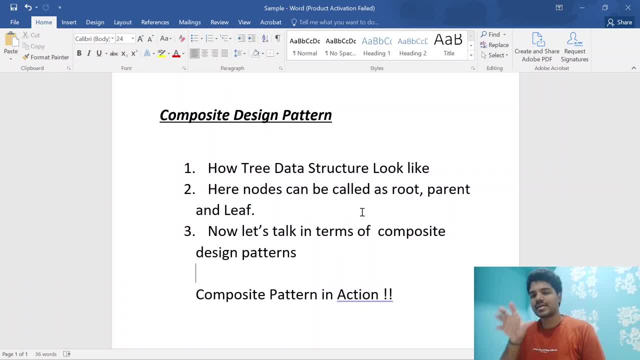 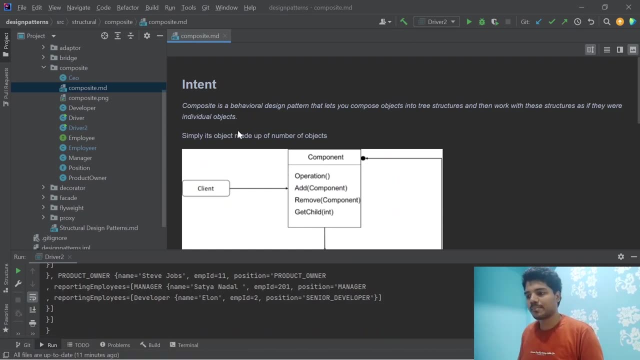 like at the bottom of tree. we don't have any sub-chails. We will basically called as, like leaf nodes. So this is the same. exact same pattern will apply to the composite design pattern also. We will look initially in a short time like: let's understand the definition of composite design pattern. 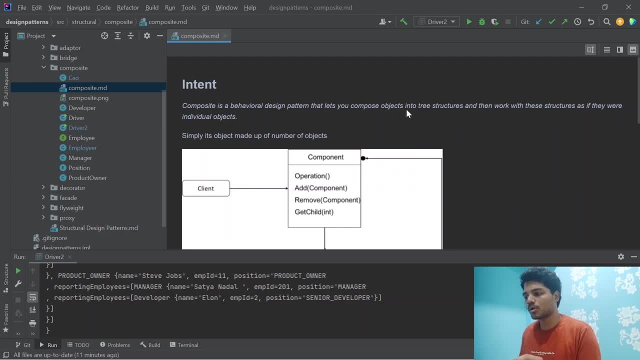 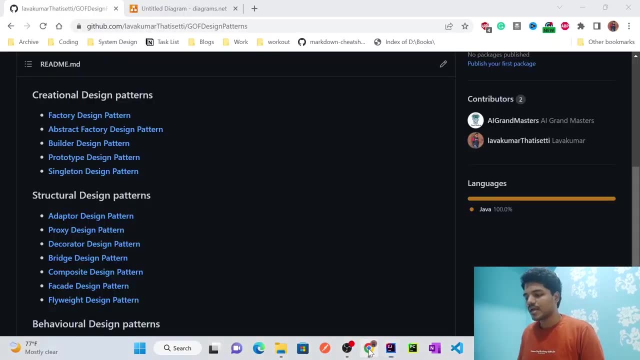 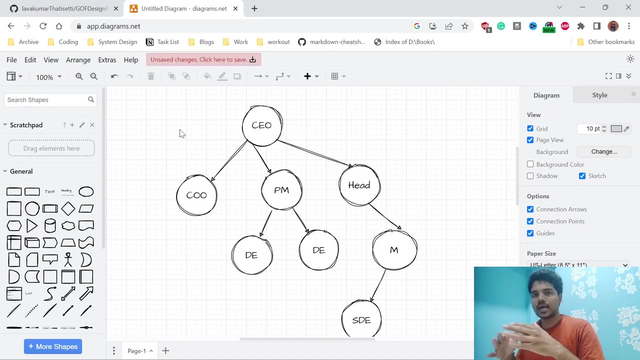 Composite is the behavioral design pattern that lets you compose objects into tree structure and then work with these structures as if they were individual objects. Which means let's say about: let's say we are in an organization where we have like a CEO and CEO has like direct reportees. 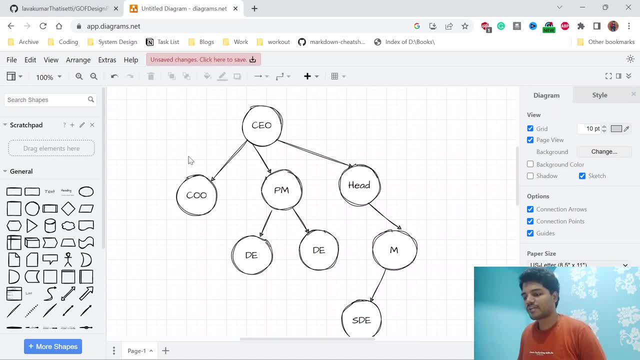 and each other reportee has like sub-reportees. And finally, there are few people who don't have any reportees. So there are few people who don't have any reportees. So there are few people who don't have any reportees, Like, let's say, there are like basically level one people. 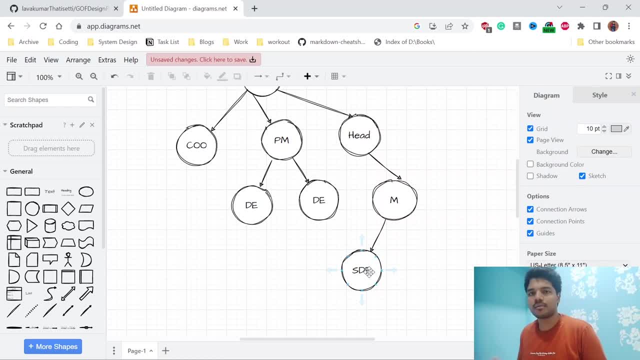 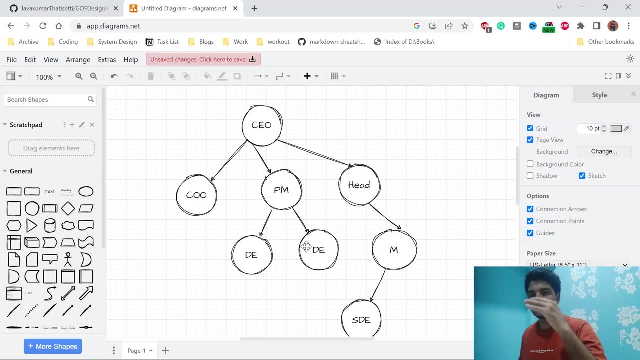 software engineers or like junior design engineers or like marketing engineers. So when we increase the each level rate, those level, those increasing levels, basically called as parent. So in the composite design patterns terms we'll basically call these four. we basically called as like leaf nodes, which is exactly we know, And these four is basically. 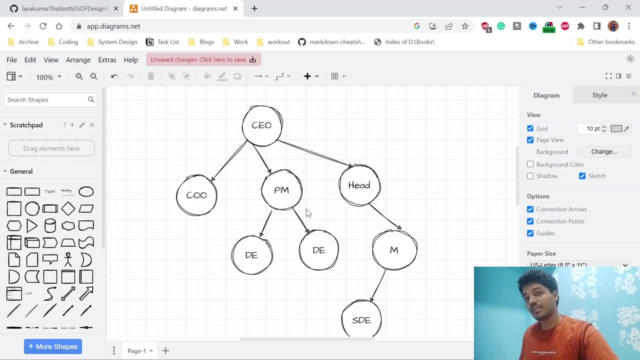 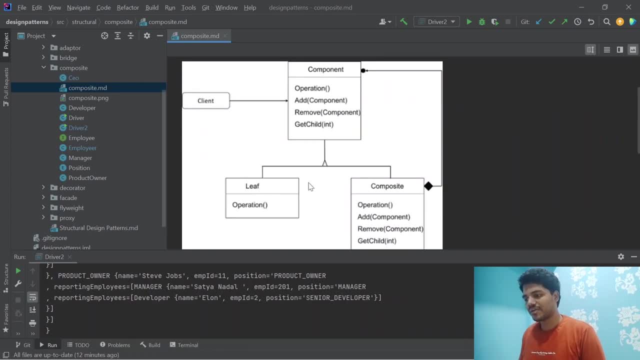 called as parents, right, And in the composite design pattern we'll basically called as like composite. if you see the class diagram you'll understand like. so we have like a leaf and we have a composite class. both are basically implement, implementing the component interface, So component. 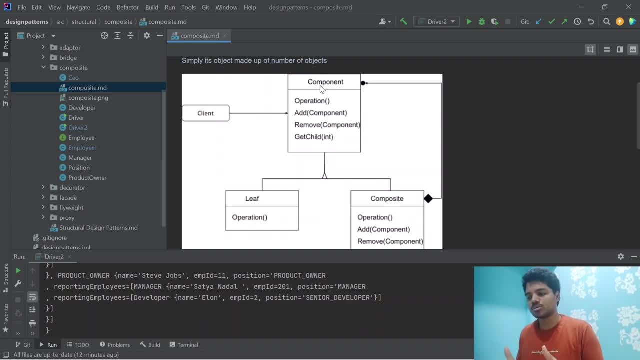 is an interface which has a common set of operations which has, like, both leaf node and composite perform. But there are a few operations where leaf node cannot be performed. Let's say adding, removing, get shell. let's say I'm a software engineer. no one is basically reporting to me. So 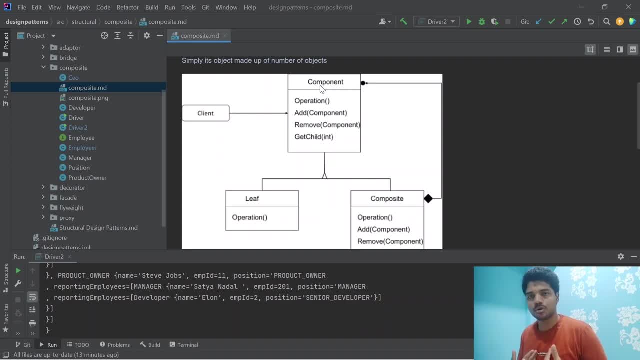 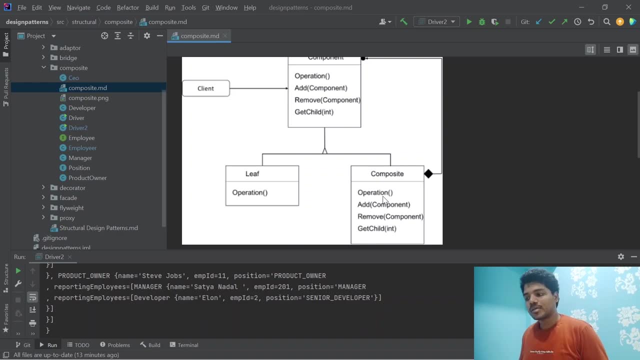 which means I basically handle components, which means I'm briefing them, which means basically I'm, I basically make a calling myself as a leaf node. so my manager: here she is basically composite class. she can add new employees, she can add renew employees, she can get the list of employees. 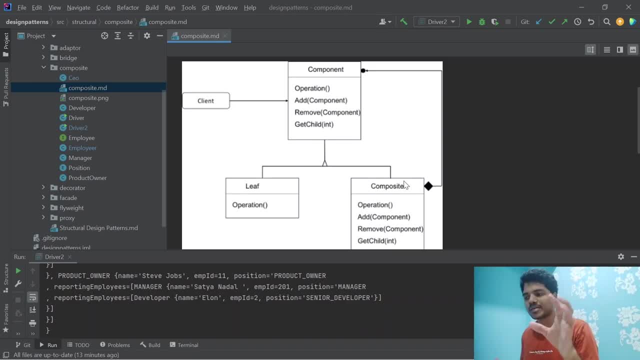 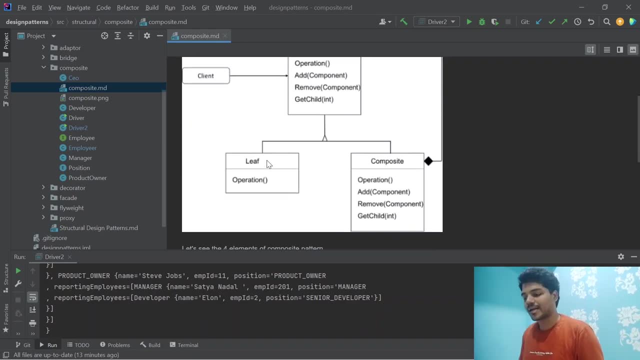 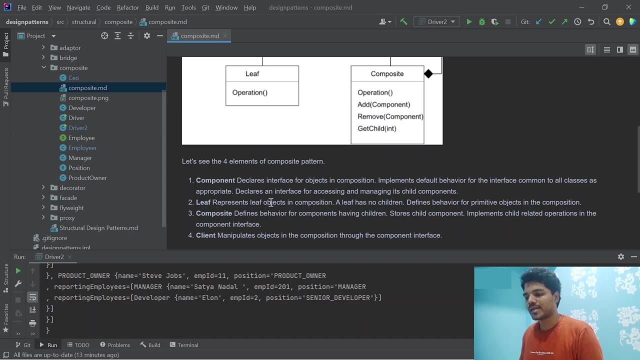 like so, which means that all the operations which are in component applies to the composite class. okay, as my manager like, so this is like general class diagram. so, as we discussed component, I declare the interface and leaf node is basically the leaf. like leaf is represent the leaf object in composition which has no children and composite defines the behavior. 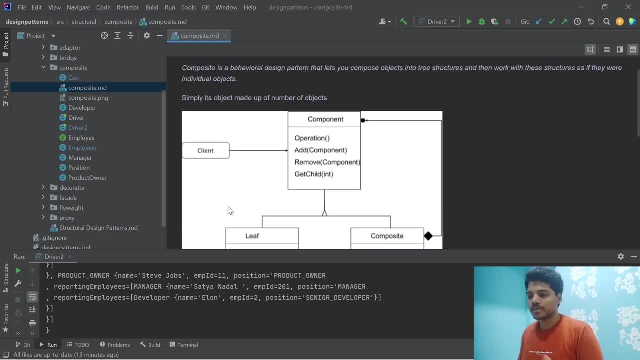 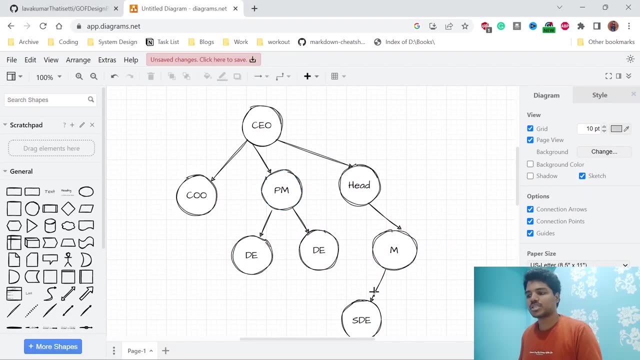 for components having children. so you can go through this particular talk. let's discuss whatever we have discussed here, right? let's convert it into the Java program. so here I will explain the two ways. one is basically each node. I will make it as like each class, right? 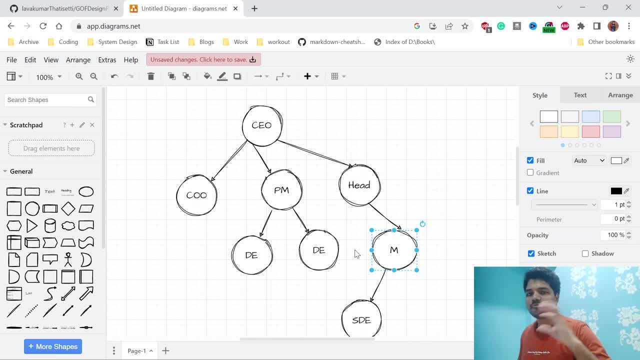 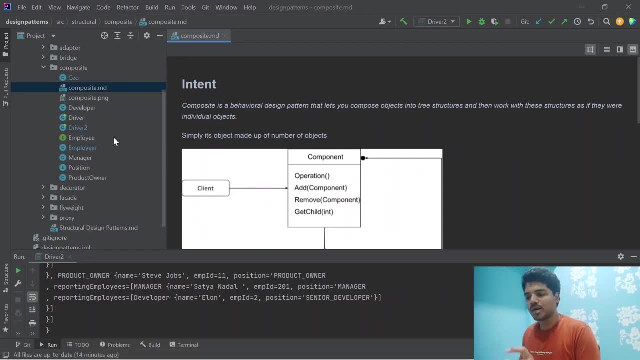 and second thing is like i'll make only one class and one leaf node. then you can understand difference between both of two. now let's say i have a, let's say i should have a component, right, i declare a component called employee. so employee has like one public function called print employee. 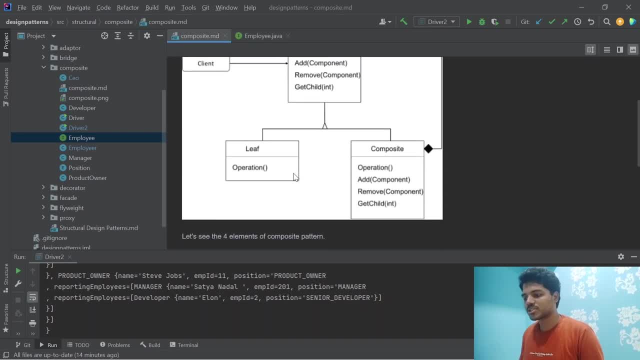 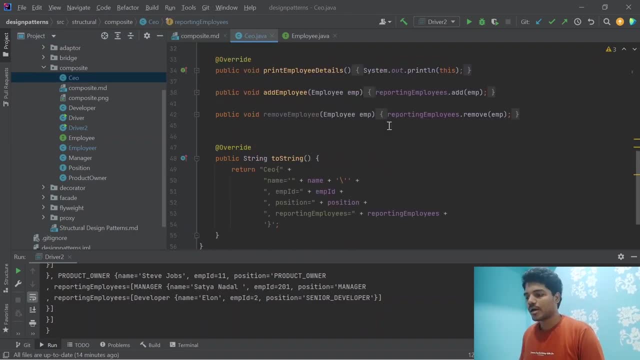 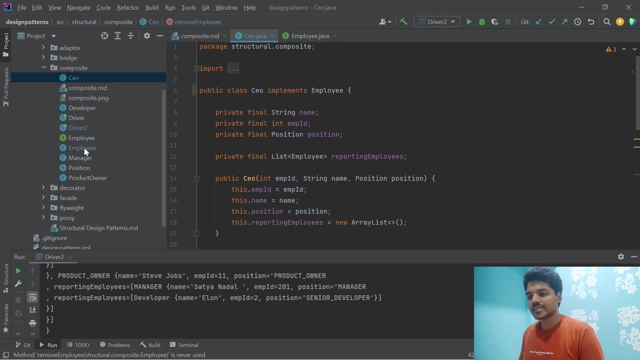 details. so let's next thing, let's talk about like composite. so i have like a ceo which is like composite class, which implements the employee. it can. it can perform add, remove and also print the employee details. similarly, ceos might have product owners also. product ones also can do add, remove operations. managers can do add, remove operations and 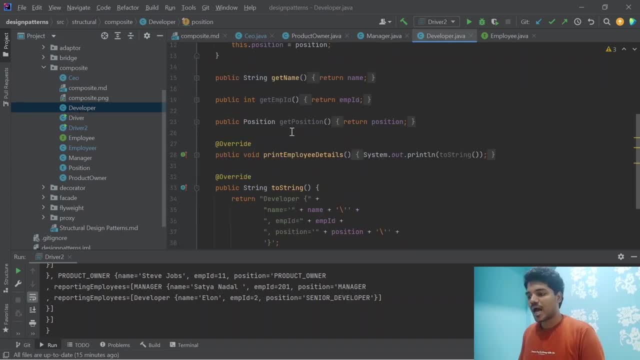 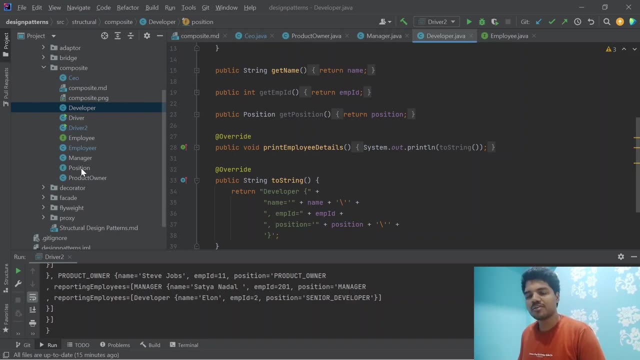 at last the leaf nodes here i'm categorizing as developers. i cannot have any add remove operations. i cannot do anything because i was, i am the leaf node like. so how can we identify like who is manager, who is ceo, through help of position enum, like uh, ceo, product owner, man, all these things. so if you 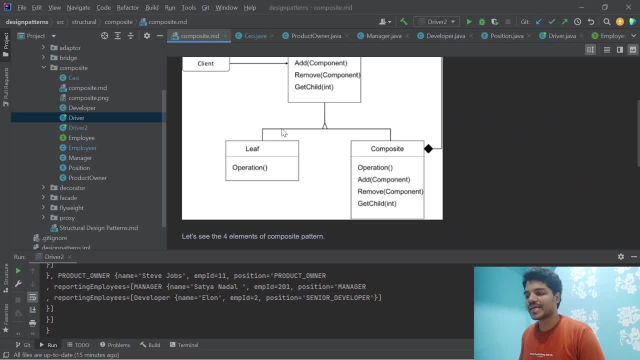 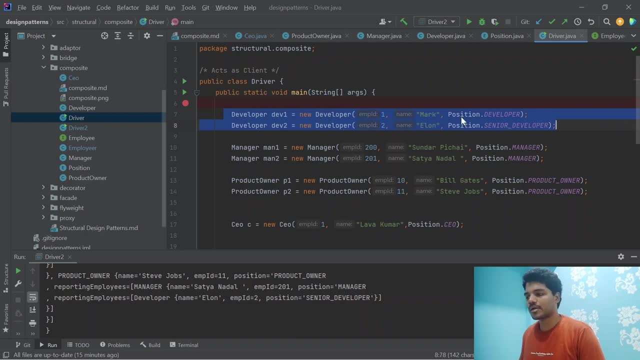 see into the driver program. basically, uh, in this diagram, basically client client code. if you see the client code here, initially i was declared two, two developers called market alone and there are two managers, sundar picture and satya nadala, and there are two product owners, bill gates and steve. 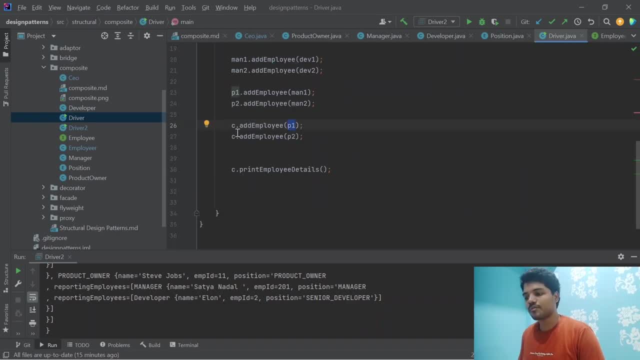 jobs and there are one ceo. that of course me ceo has, like all the employees, but ceo's direct report is basically p1 and p2 and so on. and then there are two product owners: bill gates and steve jobs is basically p1 and p2, which means like, uh, two product owners and each product owner has like. 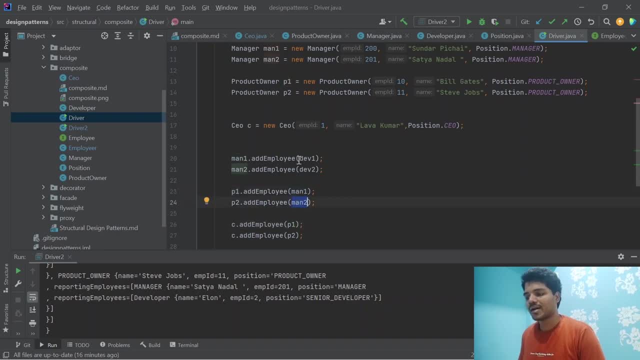 direct reporting called manager one and manager two, and manager one has direct reported dev one and manager two direct reporting as dev two. so at last dev has like in it. we cannot add anything like to the dev right, so we cannot add employee. we cannot remove employee under dev. so instead of 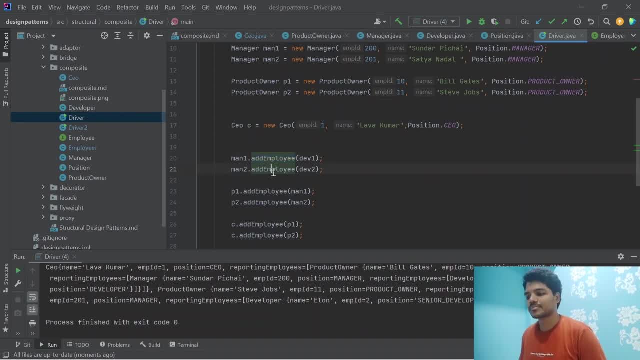 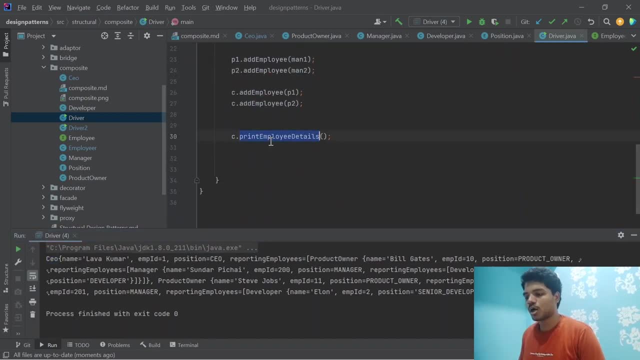 adding employee, the better way we call it as like add reporter click. so if you see here, right, if i'm getting the info details of the ceo, whenever i print the info details of ceo i'll get the complete details. so let's say i am printing the info details of like uh, um, let's say dev1 dot, uh. 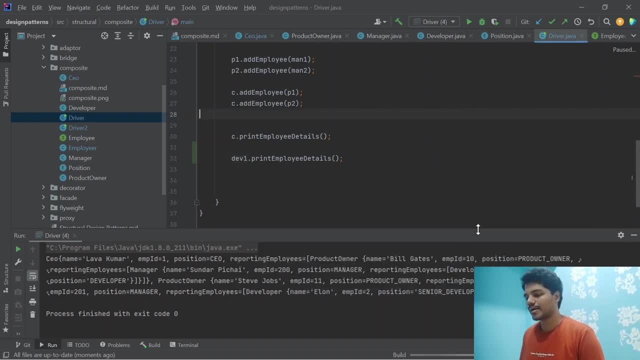 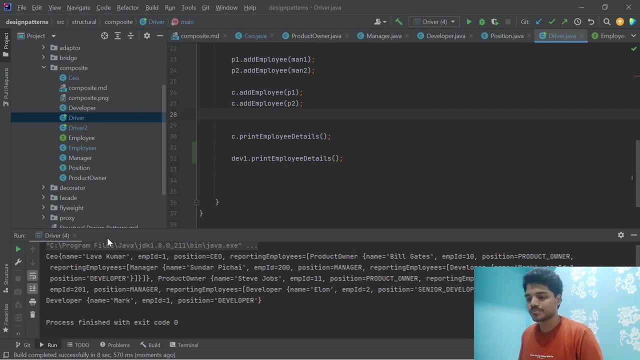 print employee details. i shouldn't get anything uh under under report is right. so that is the basic difference between the leaf node and also composite node. so developer uh has don't have any report is, but ceo has like uh, their report is called pro two product owners and dev one has like 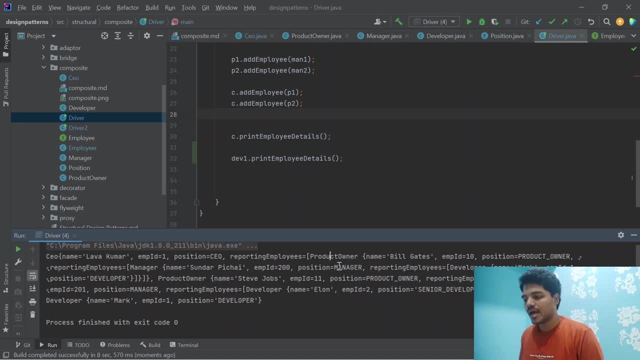 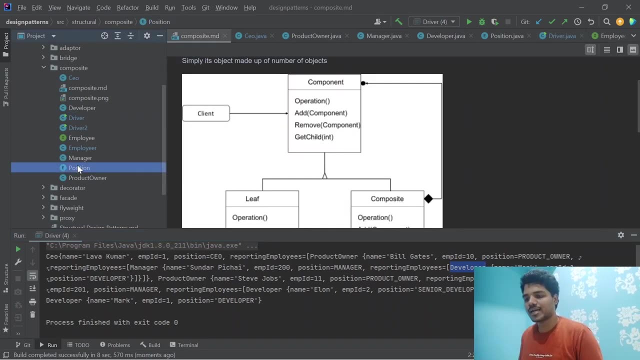 each product owner has like reporting called uh manager, and each manager has like developer. so that's the complete hierarchy. will look like it's a complete tree data structure, if you understand clearly. we have a something object called position, object uh, where we can identify uh the particular. 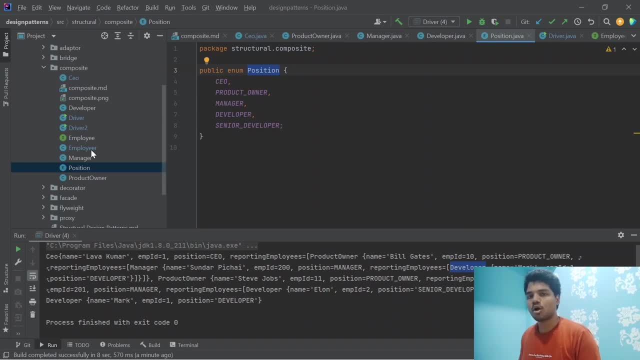 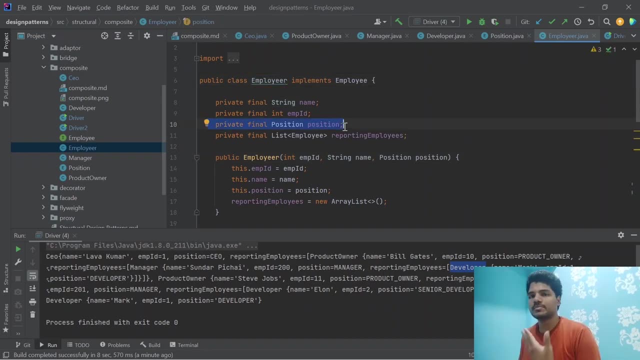 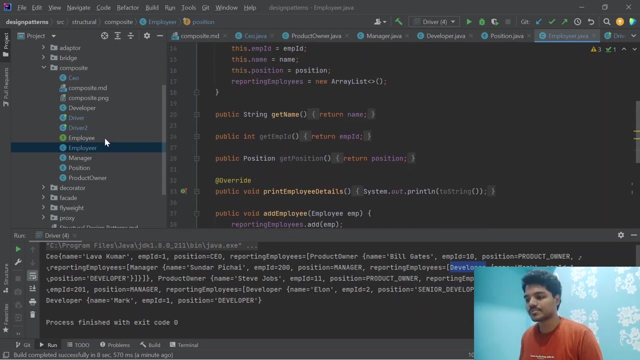 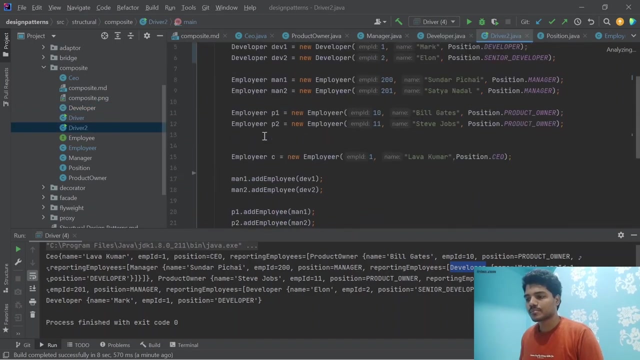 employer, right. so why can't we make a single composite object called employer? so with the help of position object i can identify: uh, who is this employee? uh, is this ceo or manager or product? this employer is basically has like add, remove and get permissions. and also let's make this developer as a leaf node. so if you see my driver 2 program, uh, so i have like,